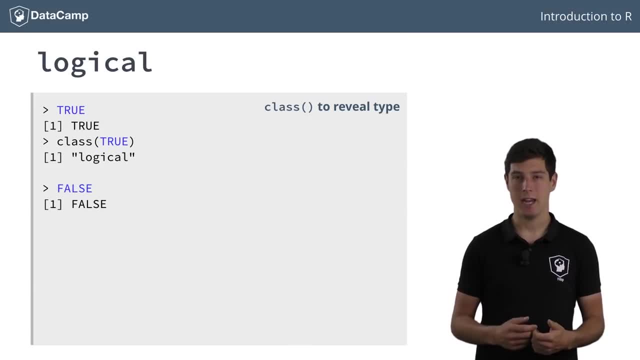 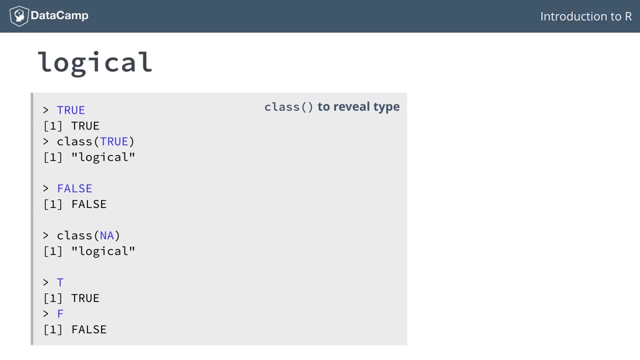 True or False. Well, actually, Na to denote missing values is also a logical, But I won't go into detail on that here. True and False can be abbreviated to T and F respectively, as you can see here. However, I want to strongly encourage you. 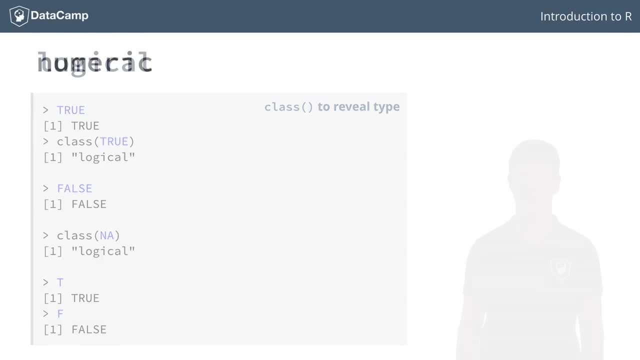 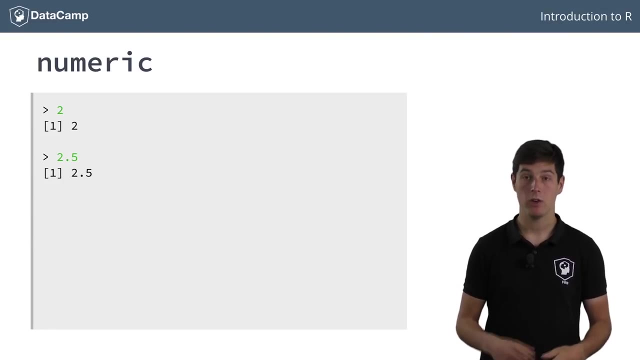 to use the full versions, True and False. Next, let's experiment with numbers. The values 2 and 2.5 are called numerics in R. You can perform all sorts of operations on them, such as addition, subtraction, multiplication. 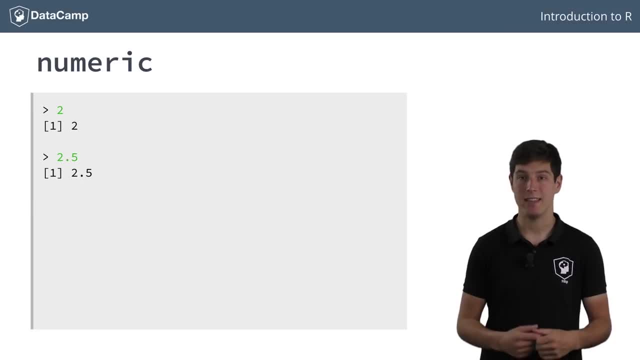 division and many more. A special type of numeric is the integer. It is a way to represent natural numbers like 1 and 2.. To specify that a number is integer, you can add a capital- L- to them. You don't see the difference between the numbers 1 and 2, but you can add a capital. 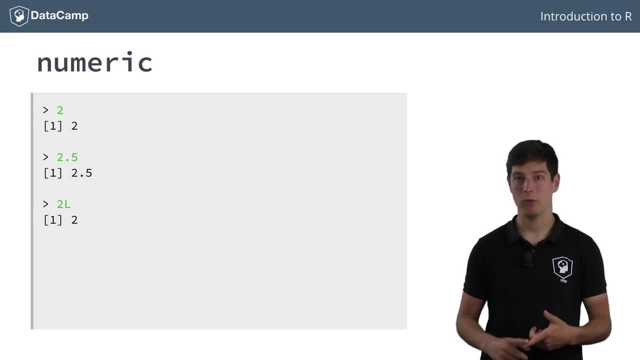 L to them. You don't see the difference between the numbers 1 and 2, but you can add a capital L to them. You don't see the difference between the integer 2 and the numeric 2 from the output. However, the class function reveals this difference. 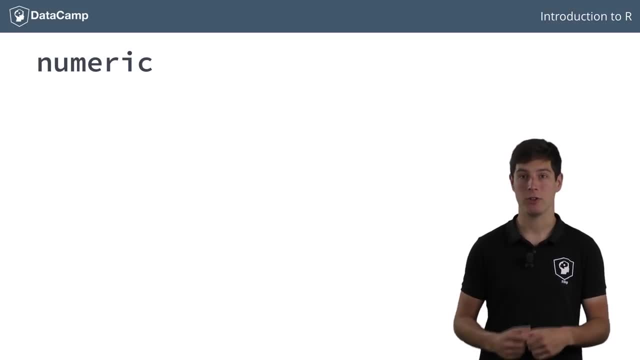 Instead of asking for the class of a variable, you can also use the isfunctions to see whether variables are actually of a certain type. To see if a variable is numeric, we can use the isnumeric function. It appears that both are numerics. To see if a variable is integer, we can use isinteger. 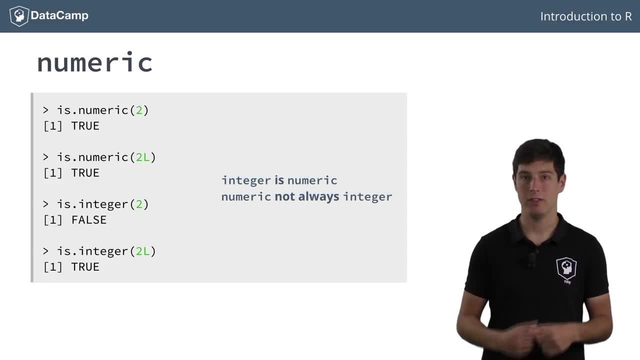 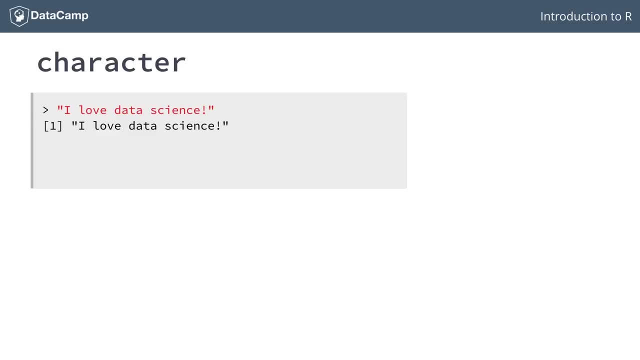 This shows us that integer is a number, but it is not a number. It also shows us that integers are numerics, but that not all numerics are integers. So there is some kind of type hierarchy going on here. Last but not least, there is a character string. 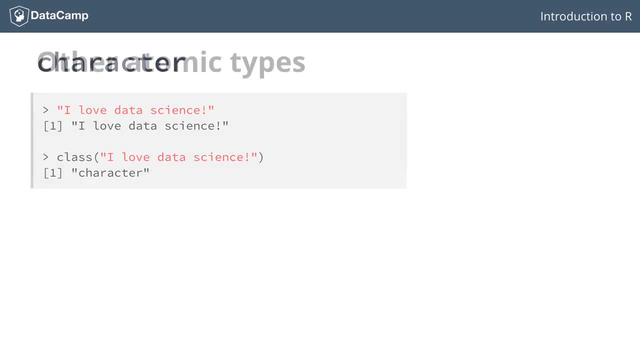 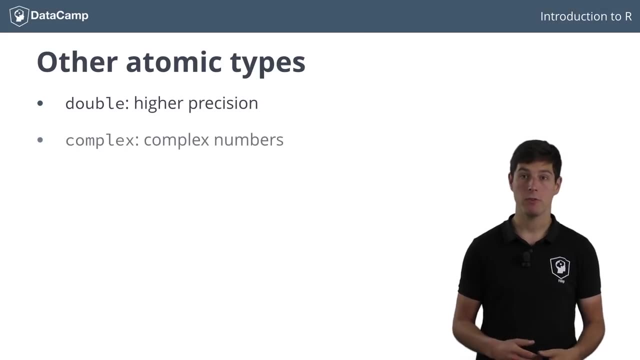 The class of this type of object is character. It's important to note that there are other data types in R, such as double for higher precision numerics, complex for handling complex numbers and raw to store raw bytes. However, you will have tons of fun working with numerics, integers, logical string and 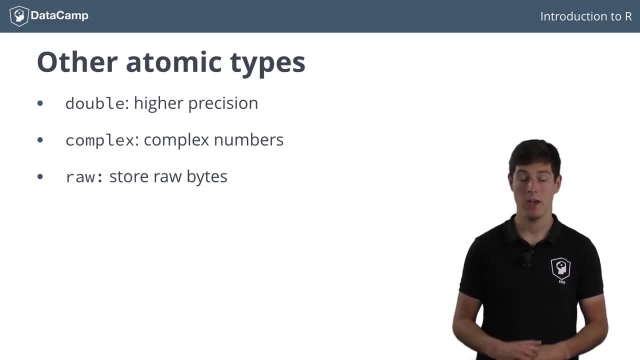 characters in the remainder of this introductory course, so we'll leave these alone for now. There are cases in which you want to change the type of a variable to another one. How would that work? This is where coercion comes into play. By using the isfunctions, one can coerce the